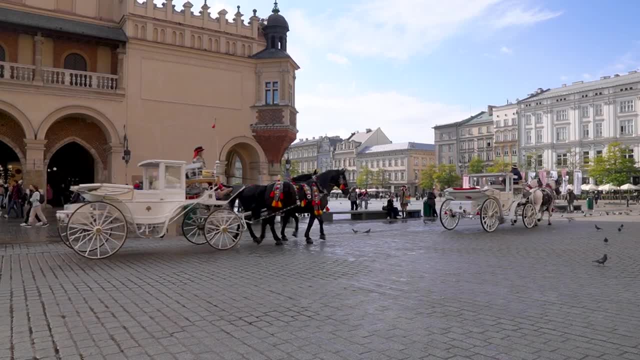 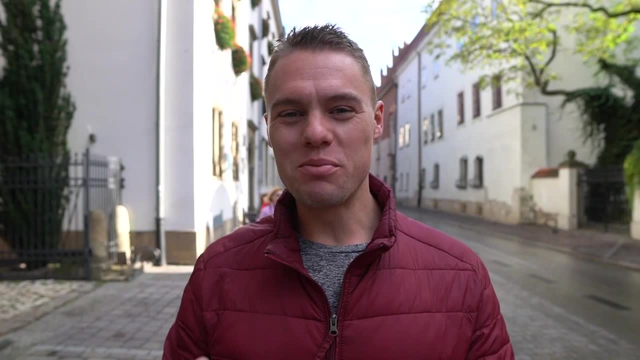 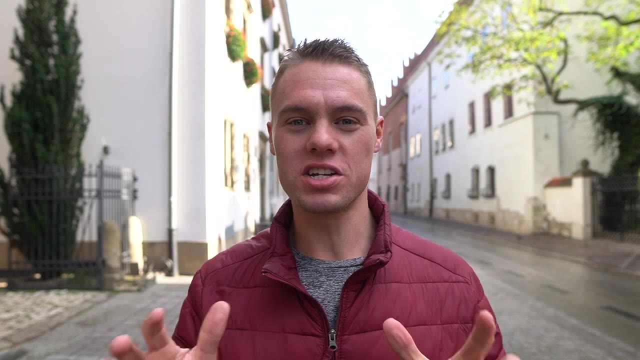 in Russia. Now, just looking at the numbers of Poland by itself doesn't really give us or you a fair comparison to what it's like in other countries, So we wanted to compare it to the United States, the country that we're born in, the country we're from, Canada, our neighboring country- a country that is known to be very safe and also the country that we've been living in for the last six years: Mexico. Starting with Mexico, This is the homicide rate per 100,000 people. The homicide rate in Mexico per 100,000 people is 26.. 26 out of 100,000.. Like I said, that's a country we have. 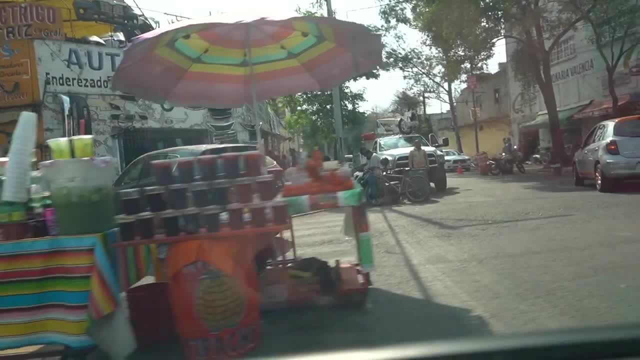 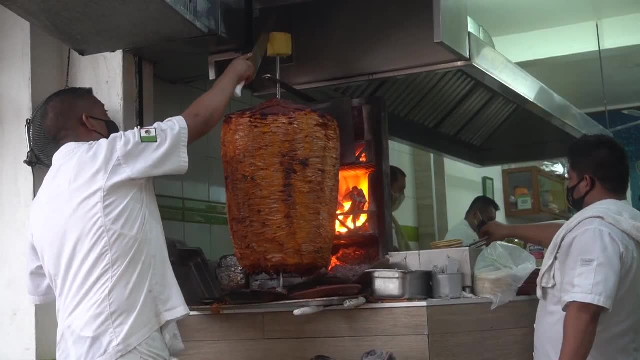 lived in for the last six years and have. it wouldn't be a place that we lived unless we felt like it was safe enough for us to live there, And we've traveled around the whole country so we've felt like it's pretty safe. But compare that to the United States, which has a homicide rate of 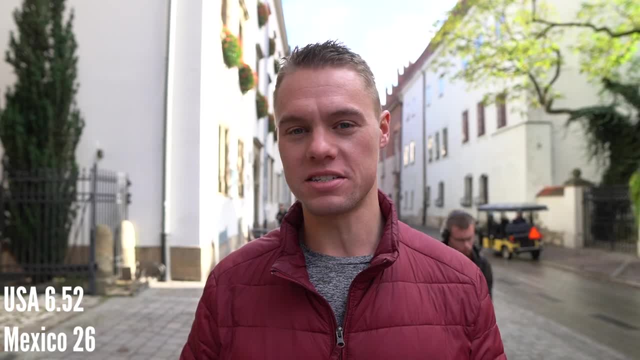 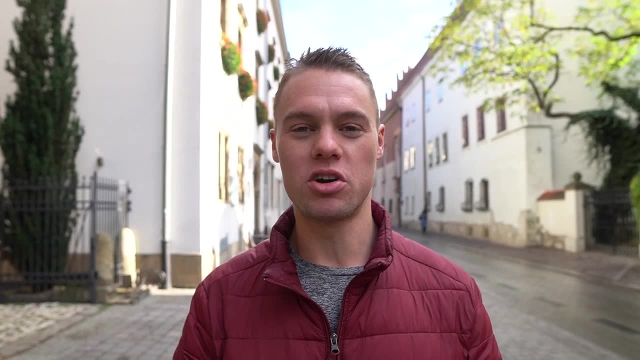 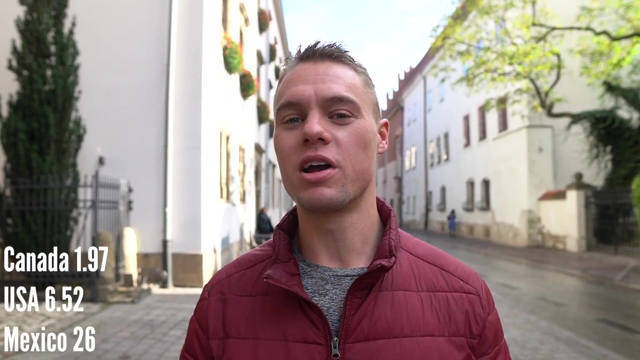 6.52 per 100,000. So considerably less than Mexico. But then we moved to Canada. Now the Canadians are proud, very proud of their safety, very proud of their country, as they should be. They have a homicide rate of 1.97, a third of the homicide rate that we have. in the United States. So that's a pretty good number. But compared to the United States. we've traveled around the whole country so we've felt like it's pretty safe. But compare that to the United States. we've traveled around the whole country so we've felt like it's pretty safe. But 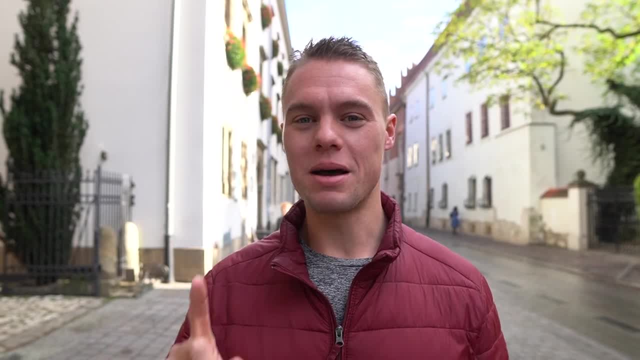 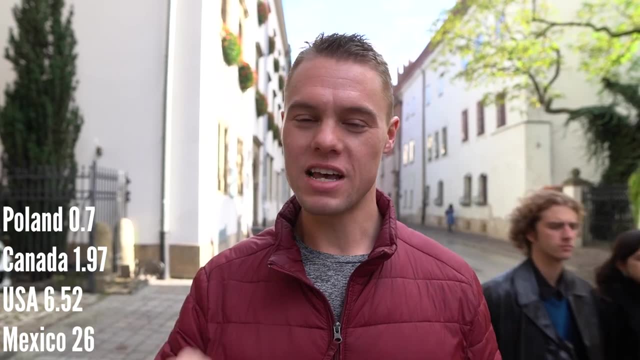 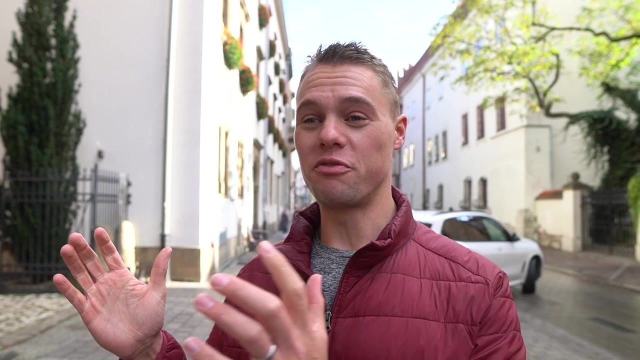 Poland. the homicide rate in Poland is 0.7.. Not 1.7,, not 5.7, 0.7.. 0.7 per 100,000 people. Those are the numbers. Like I said, we felt safe in the United States. 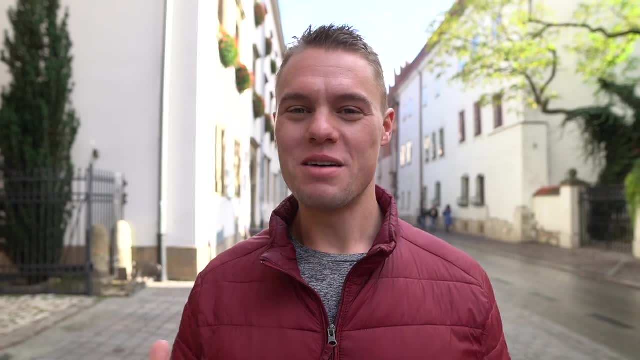 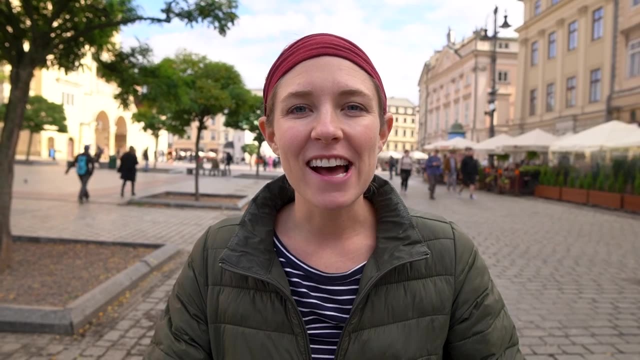 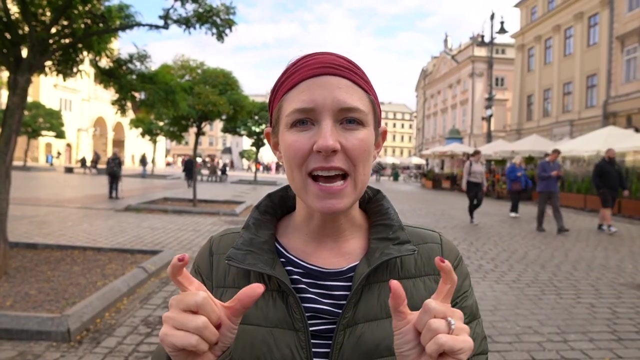 We felt safe in Mexico. We have never been to Canada, But you can't dispute the numbers. Numbers and data are great. As an accountant, I love the cold hard facts. But the truth is only looking at numbers and data don't really paint a full picture as to whether Poland is safe. 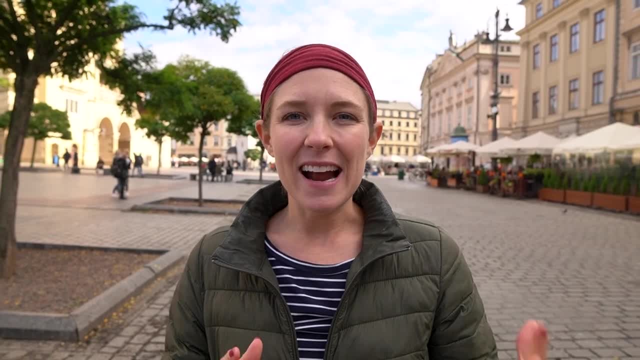 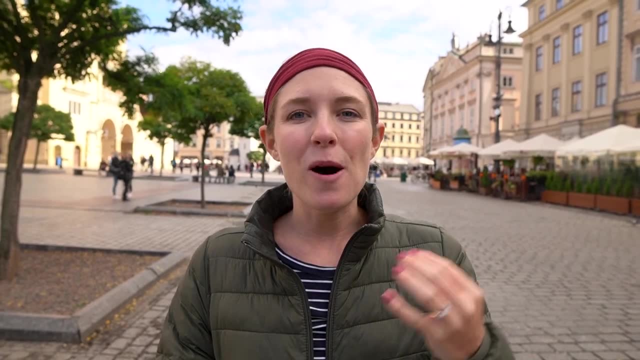 or not. So the second sort of pillar that I'd like to talk about is your spidey sense, That's what I call your intuition, that feeling in your gut about whether you feel safe in a place, And really I think we all know that feeling. you get in the pit of the road, You get in the pit of 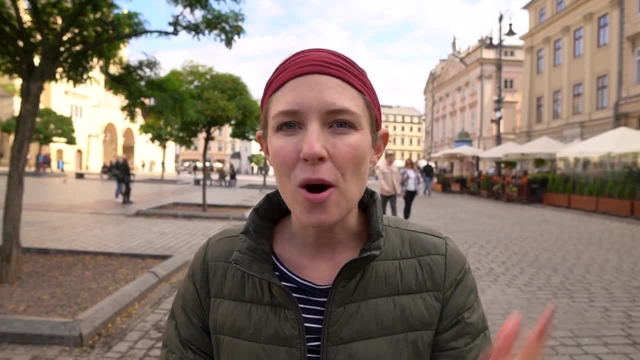 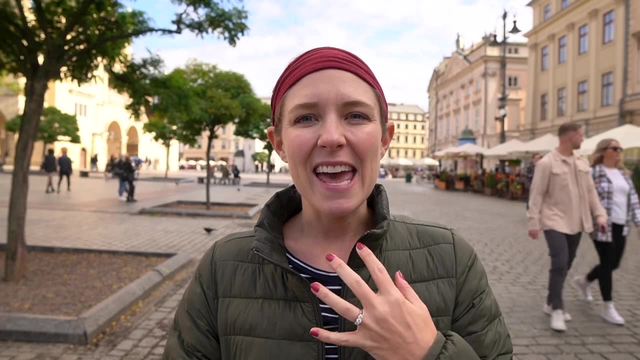 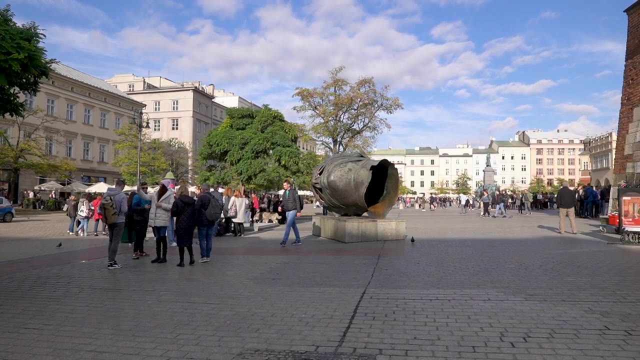 your stomach. unfortunately, when you turn down a street, you're all by yourself and maybe things feel a little off, And that, to me, is what I call my spidey sense. And what do I base that on? I think you can base that on looking at your surroundings and deeming whether Poland is safe. 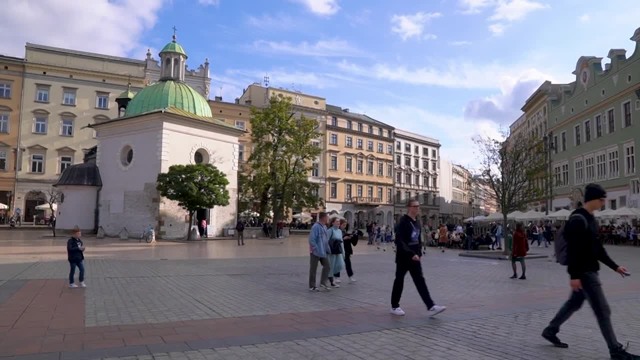 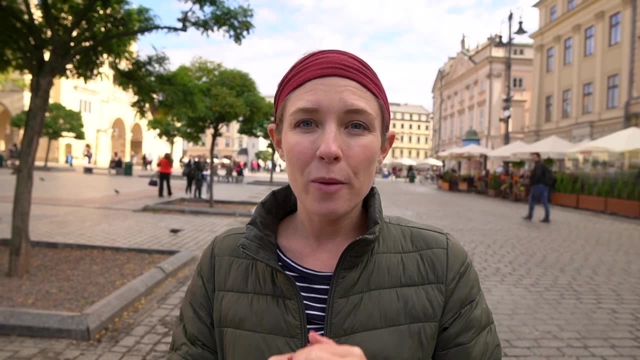 or not? Is the plaza busy or is it empty? Are there people out enjoying the time, having a great time, Or does it feel a little bit off, perhaps a little deserted? Are there bars on the streets? Does it seem like shop owners and restaurant owners are worried about break-ins or 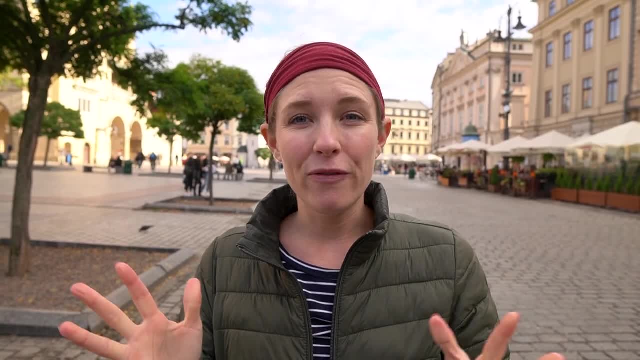 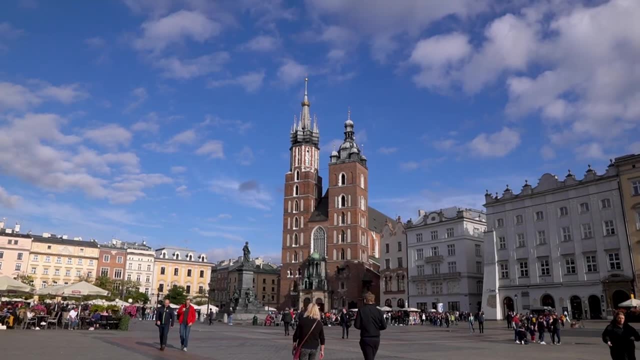 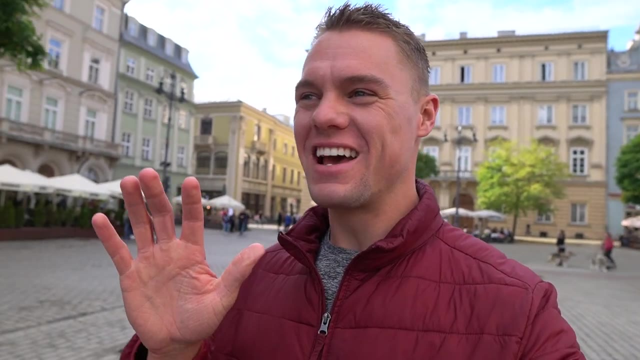 petty theft or things like that, And I would like to say with full confidence that Poland feels extremely safe, according to my trusty, spidey sense. Quick disclaimer, before we jump too far into this, is that this is based on our experience in Krakow. 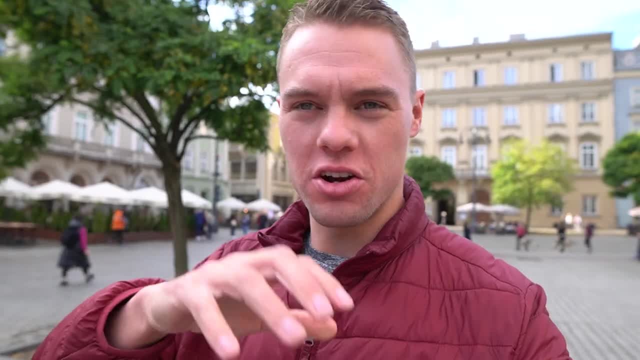 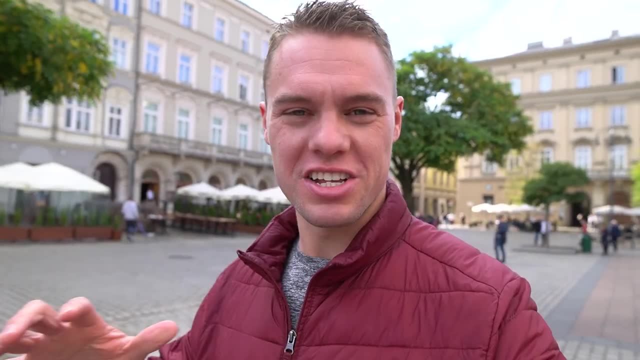 Poland. We haven't really traveled much out of Krakow or really southern Poland. We are not war correspondents. We are not Ukraine slash Russia specialists, by any means. This is purely based on one, some facts and figures, and two: 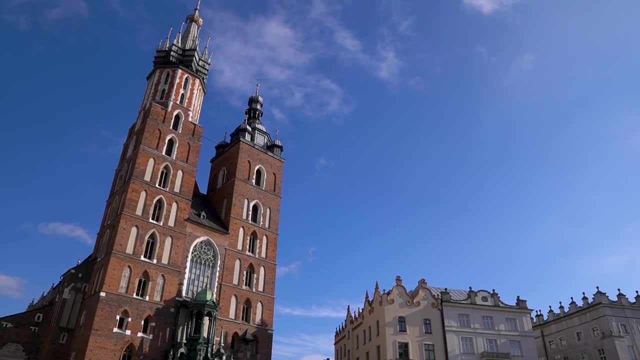 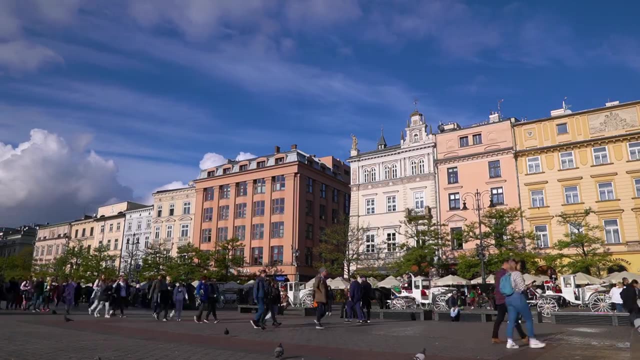 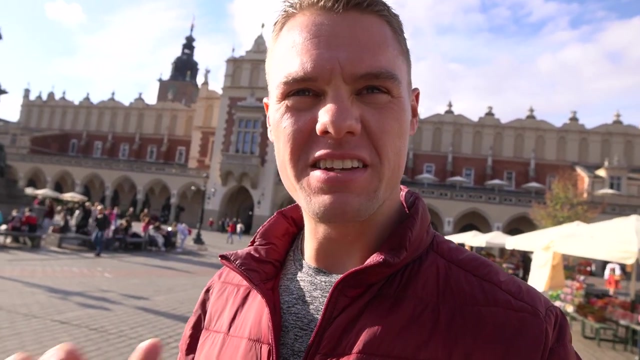 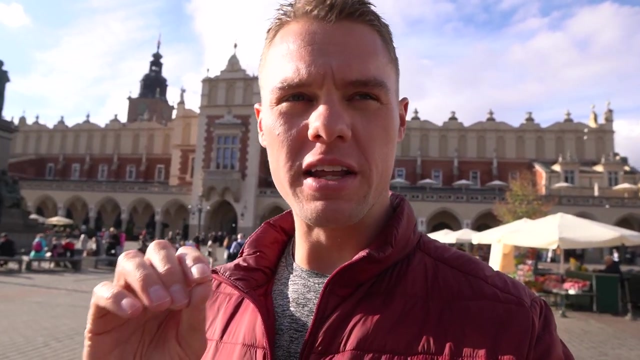 our experience in Krakow, Poland. The short answer is: we feel extremely safe in Poland. We don't feel like we're in any danger. We feel like it's safe to travel here. However, I will say there are definitely some things that make us feel uneasy. 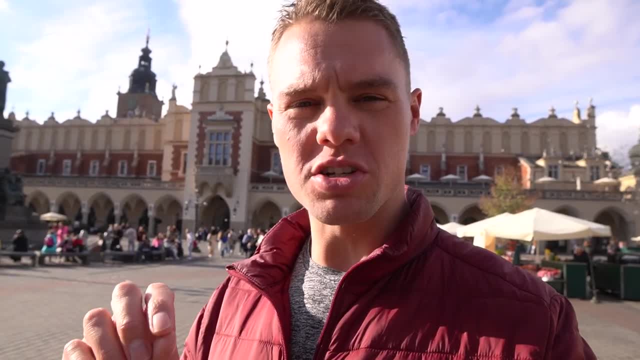 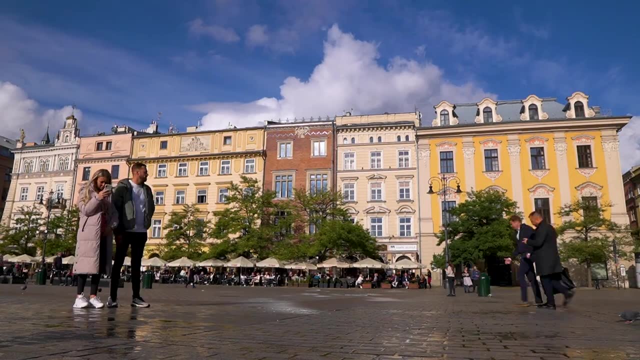 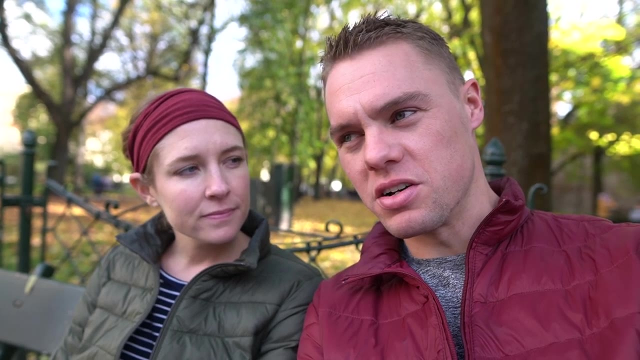 and Krakow does have some dangerous aspects to it, And we want to share those with you at the end of the video. Most people that are wondering if Poland is safe right now or not probably are thinking so in the context of Russia and Ukraine, because Poland is very close to Ukraine, It borders Ukraine. 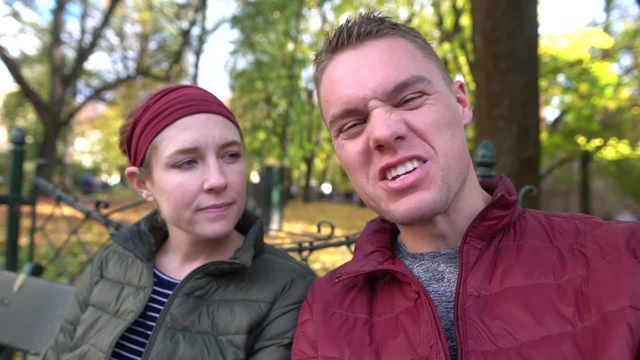 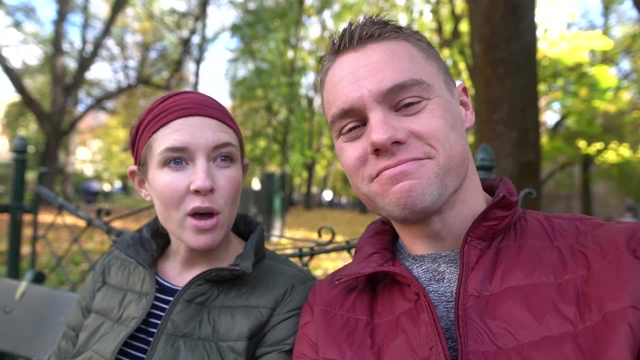 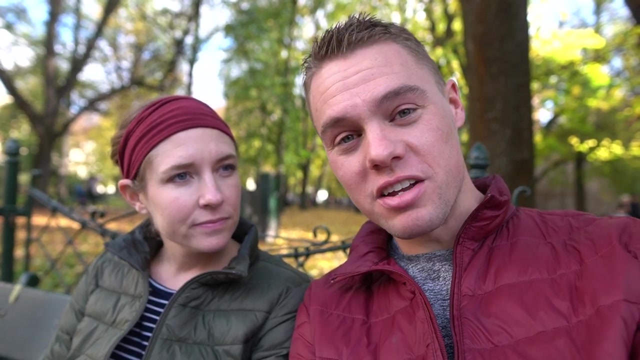 Let's keep in mind: here we are YouTubers, Not historical YouTubers, not news YouTubers. They're coming to us for war information, Abort. It's your fault, I'm sorry. Here's my view, my slightly educated view, on the situation with Poland and Ukraine: slash Russia. 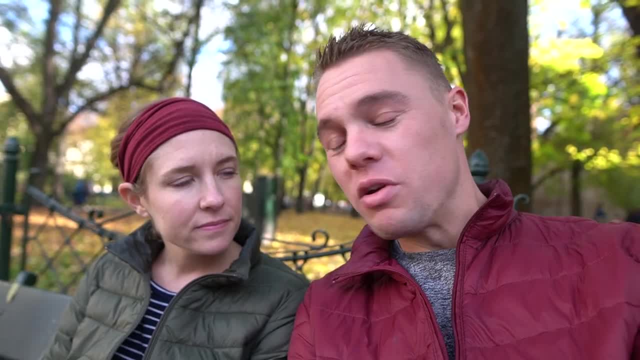 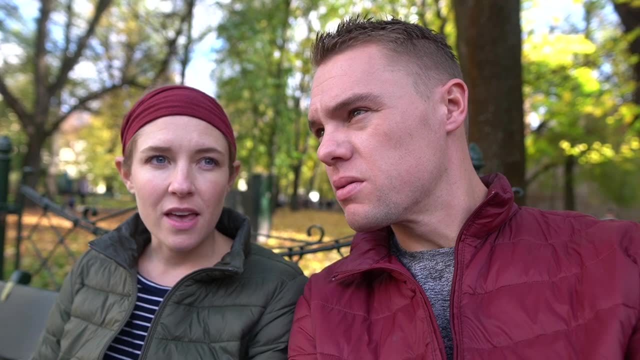 Is Poland safe right now? as of the time of this filming, We feel very safe in Krakow As a tourist. in Krakow, everything seems as it would normally any other time Again, I feel like this is with a million disclaimers. 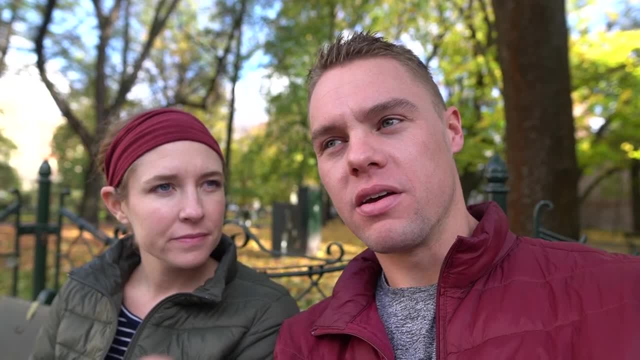 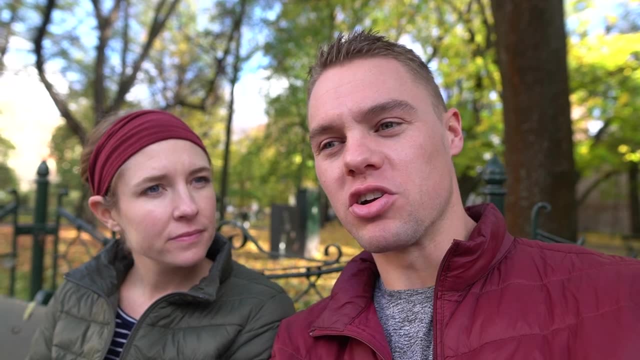 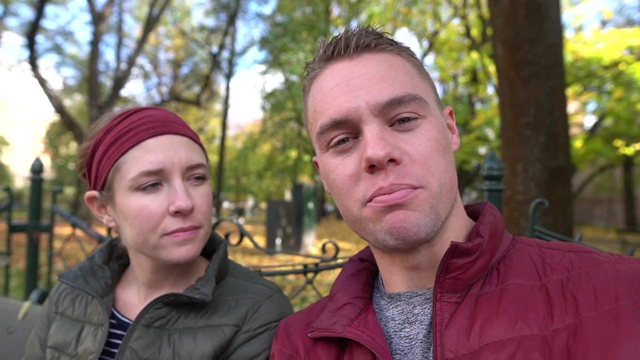 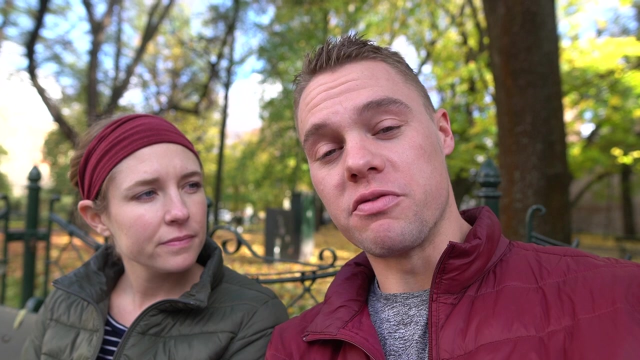 I think most people's concern or fear with Ukraine slash Russia is the unknown. It is all of the posturing. It is Russia saying they're going to do this and that And with Poland being so close to Ukraine, fears about if things were to escalate beyond Ukraine. the proximity to Poland seems fearful. 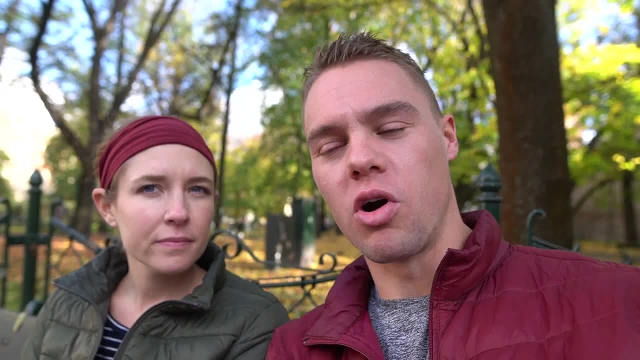 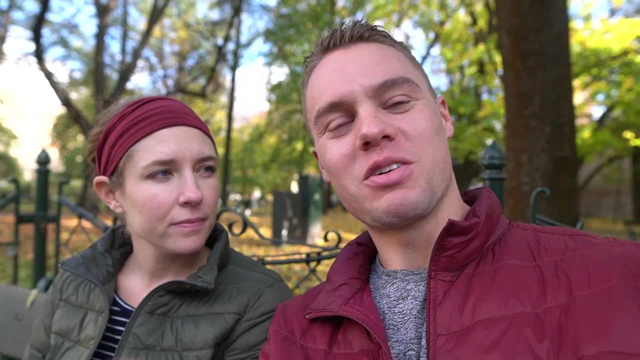 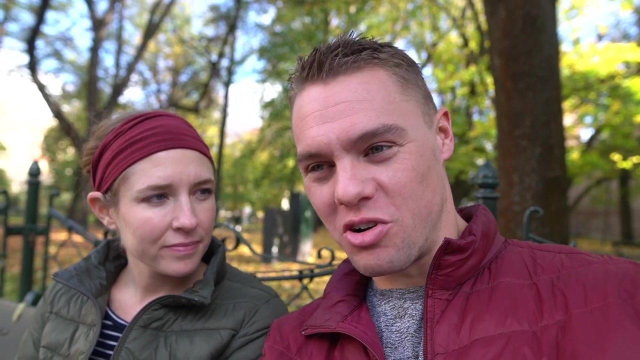 to some, to many, Especially, almost, the further away you are, I feel like, the scarier it seems. My take my view, and again, remember, YouTuber, not historian, not an expert, is that if things go beyond Ukraine, if things were to spill over into NATO, 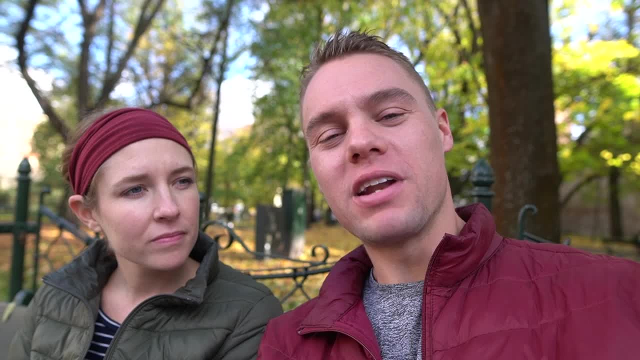 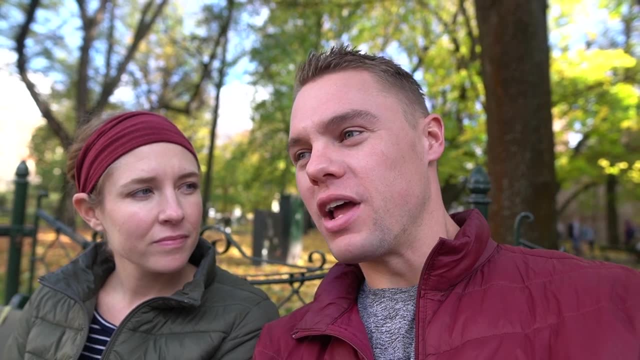 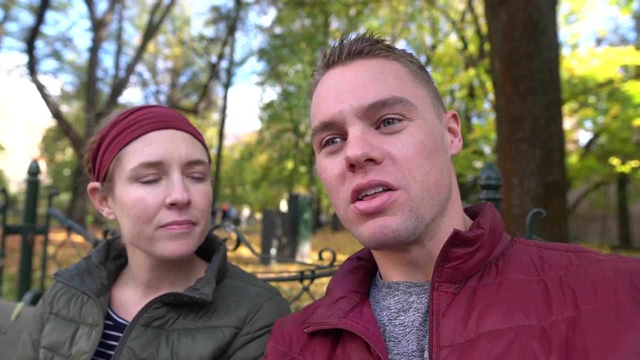 countries, we're not safe. We're probably not safe in Texas, and we're probably not safe in Poland And NATO countries. I guess what I'm trying to say is, if things escalate beyond the borders of Ukraine, then I think everybody's safety across the whole world is probably. 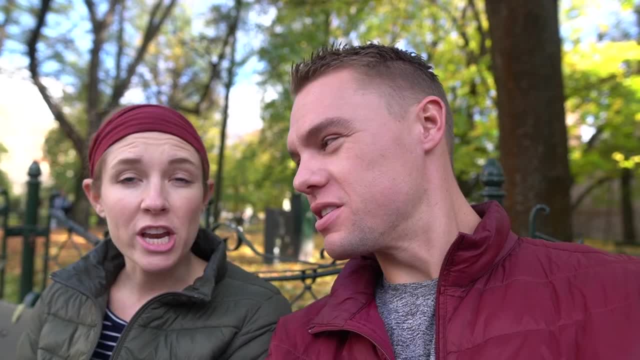 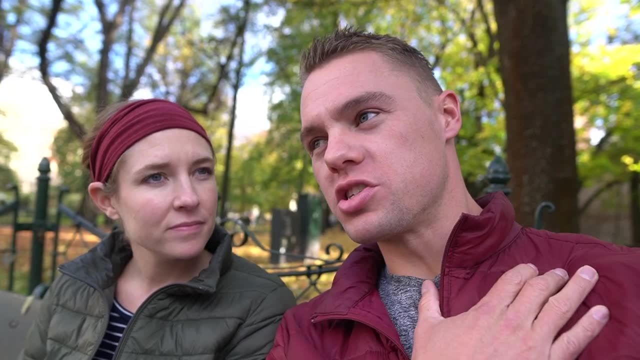 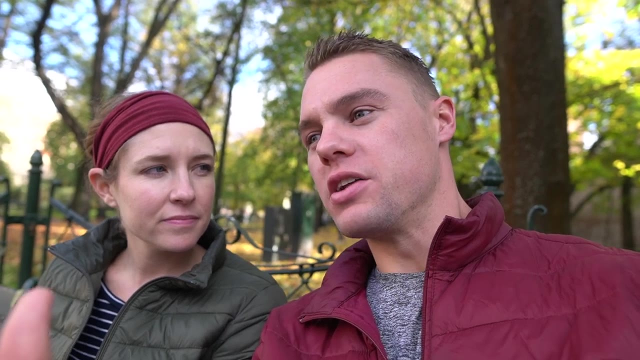 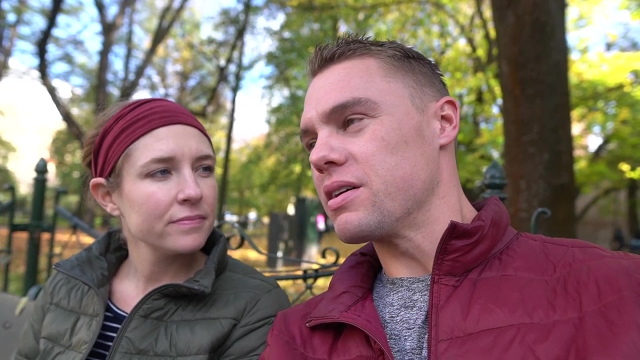 probably at question Changed, It's changed. Does that make sense? That makes sense. So I feel just as fearful here in Krakow, Poland, about the situation in Russia as I do if we lived in Dallas. That's my opinion. That is, again, not an expert. Haven't read everything about the war. 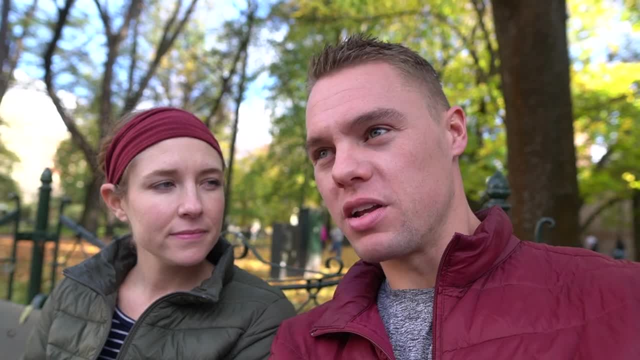 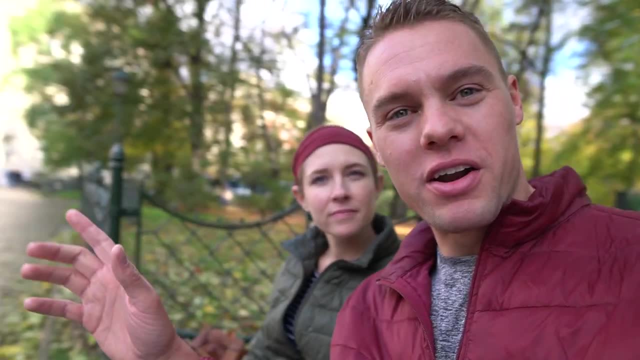 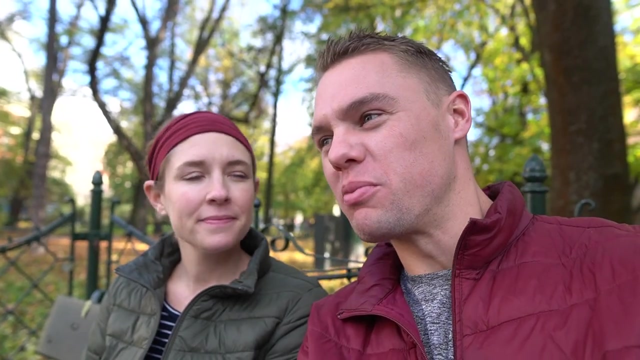 Don't know everything about the war, That's just my opinion. I'm sure many people feel differently. but I'll go back to there's people out here on scooters. There's people Dangering up the place. There are people here having fun. There are people out getting drinks. There are people from the UK. 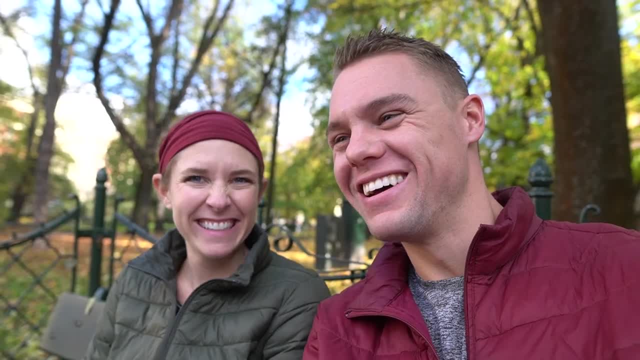 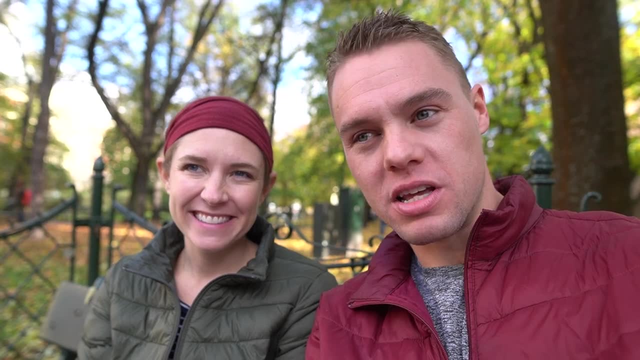 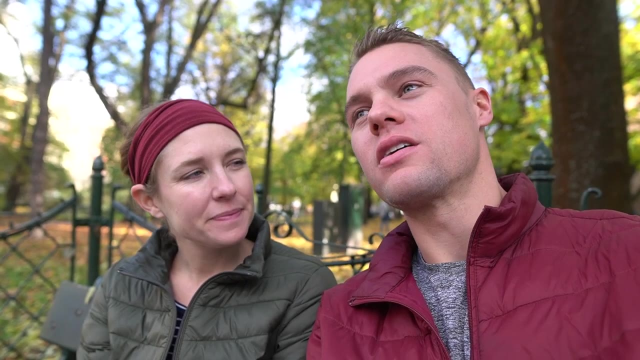 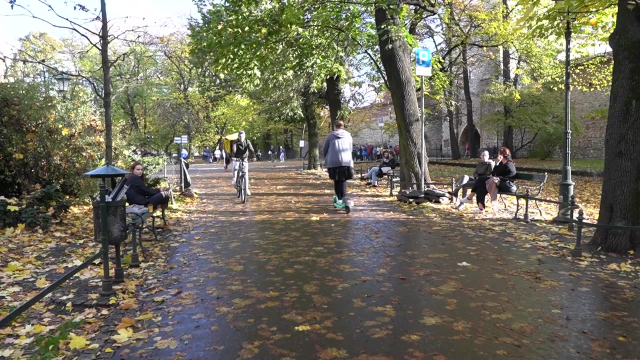 visiting here on holiday on stag parties, we've been told they're called. There are lots of tourists here, so we are not the only ones that feel like the situation in Ukraine and Russia is not a threat currently, as of this filming: Dangerous, Not dangerous. Dangerous, Dangerous. 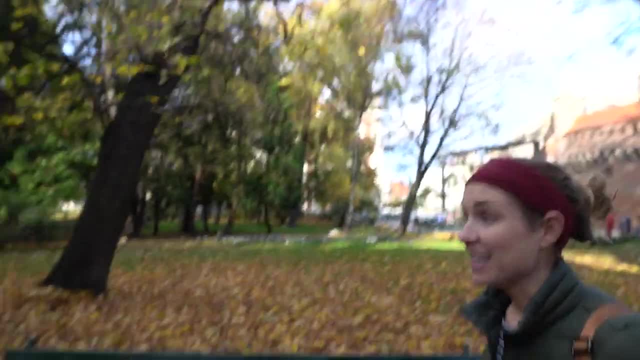 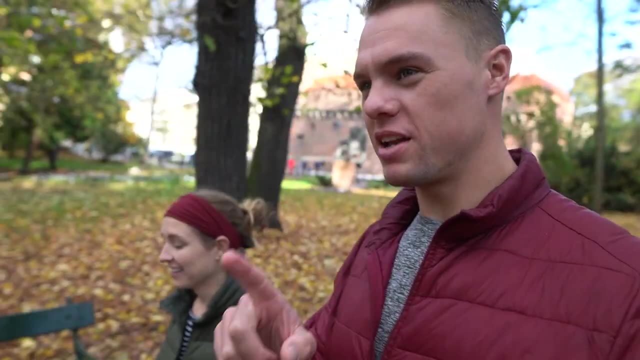 Wow, You are very passionate. You stand up for very important scooter causes. If I'm on the city council of your city, I am banning all scooters. Not if you own a scooter- Cool, It's the stupid rental scooters. 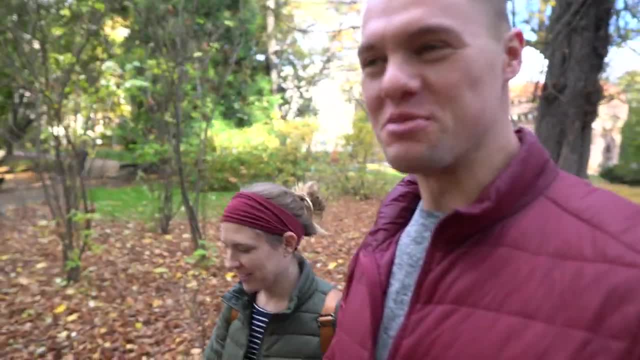 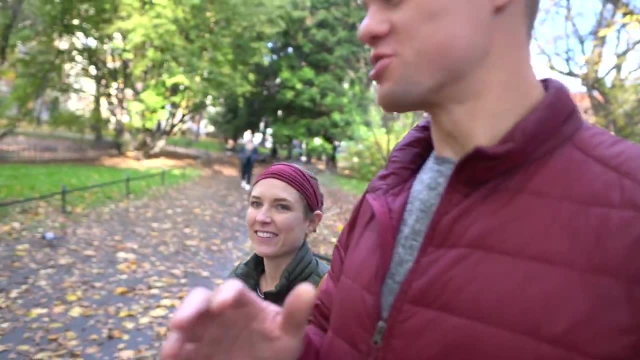 Don't get me wrong here, and probably two videos and like two videos from now. we're going to rent one tour and it's going to be a lot of fun and I'm going to love it, but I've committed to not liking the scooter so I got to go with it. Ride or die. 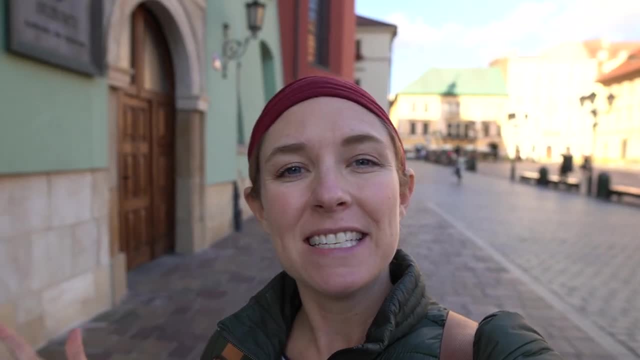 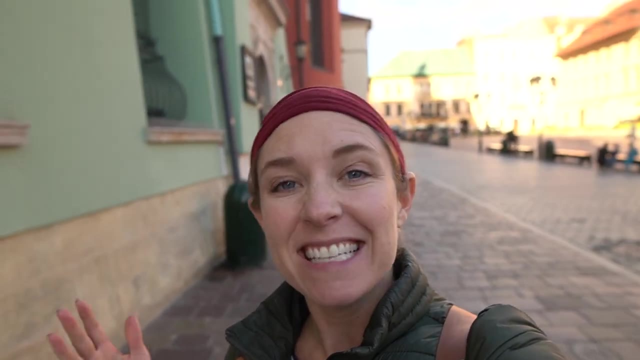 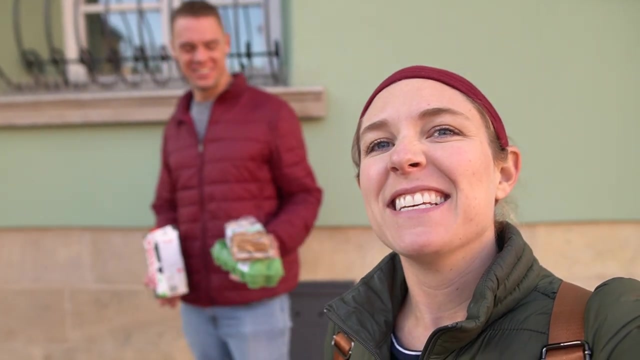 There you have it. Based on the data- the numbers are Spidey senses- and our opinions On the circumstances with Russia. we believe Krakow, Poland, is indeed a safe place. Here's what's happening behind the scenes. I feel the need to pan over here. We have eggs and milk. 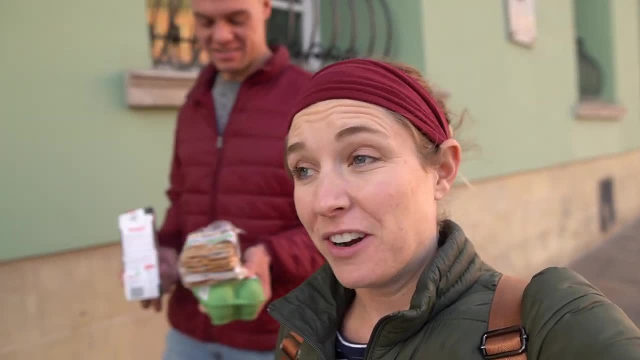 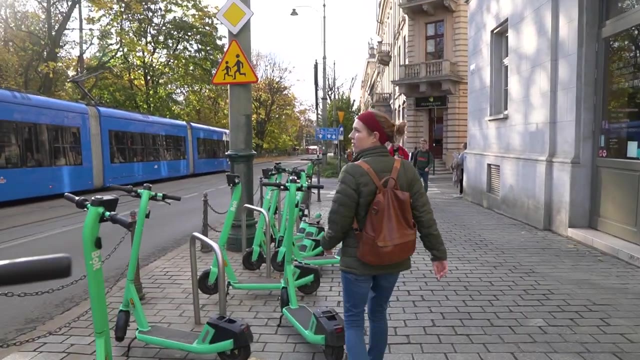 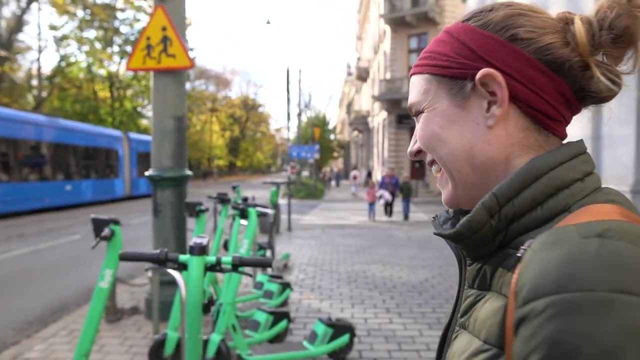 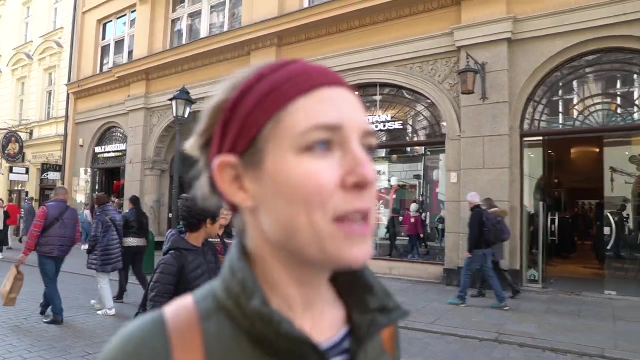 and bread because we're making tuna for dinner. That could also turn Krakow potentially dangerous. Oh Greg, These are so dangerous. How did I do Dangerous? Look at that. She just cut somebody off. Now you're making me hate scooters. I used to not have anything. 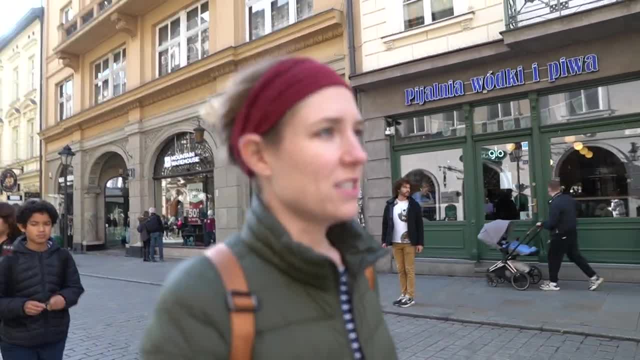 against scooters and now I just feel so prejudiced against them and I don't like it.